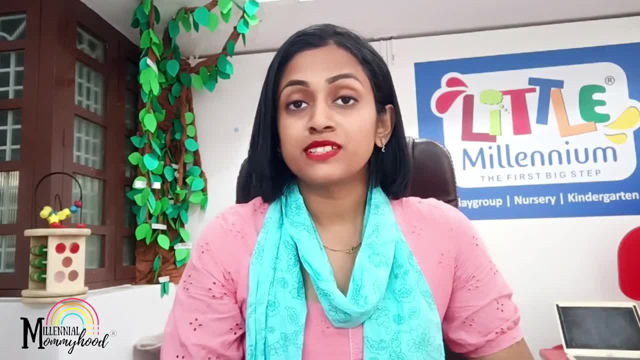 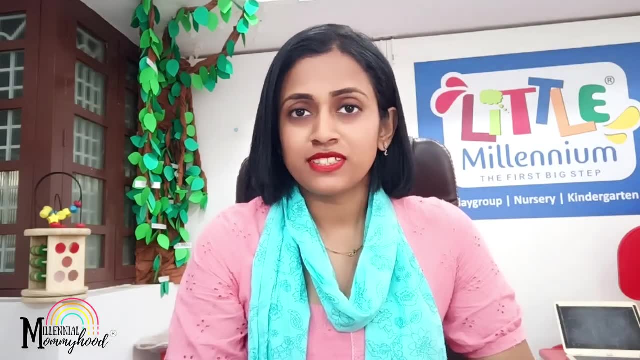 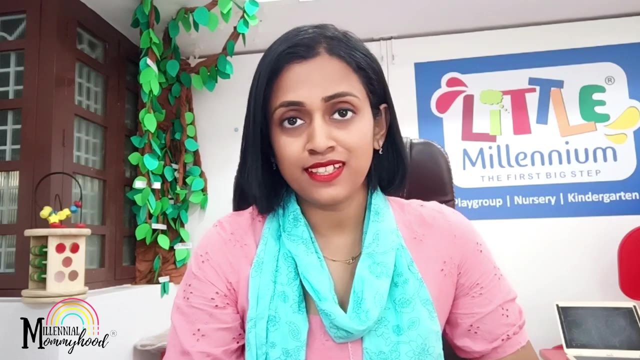 Good morning everyone. Welcome back to my channel. In today's video we are going to discuss about the right age for your child to join a preschool. So the Indian preschool system basically have four categories. It starts with playgroup. We also call it as pre-nursery. 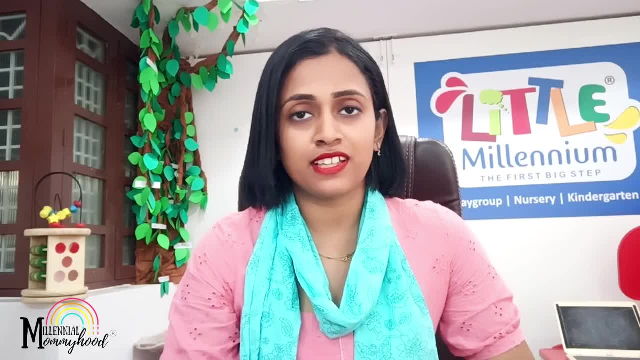 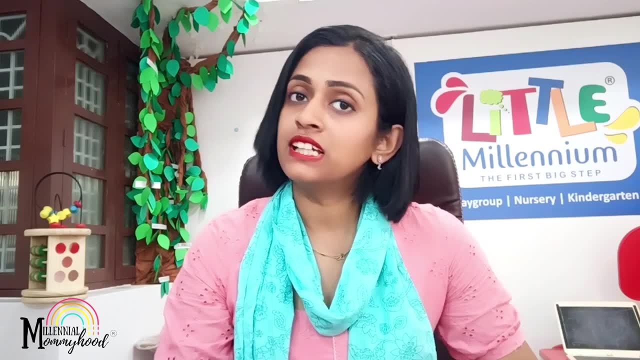 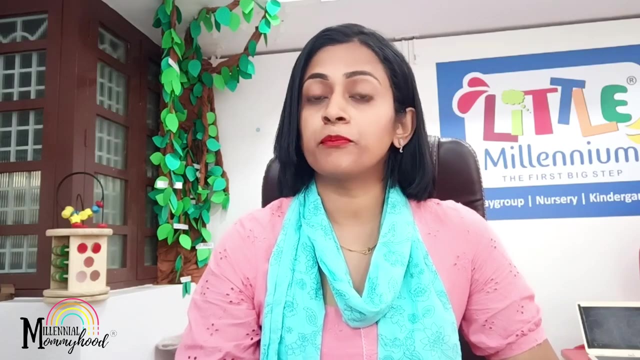 Then comes nursery, LKG, UKG and, finally, the child is ready to go to first standard. Earlier, there was no set rule for age criteria when it comes to these kindergarten classes, But now, with NEP 2020, it is mandatory that the child covers a complete age in order to be. 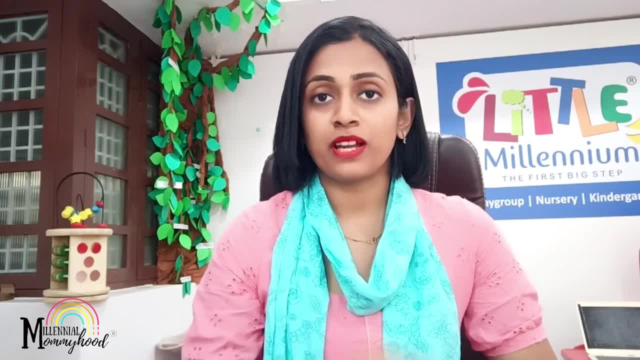 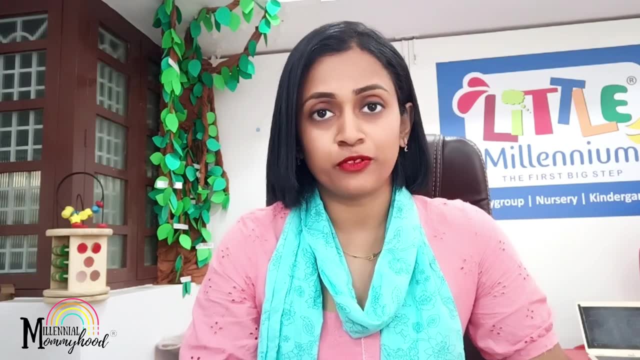 eligible to join first standard And that is how I am going to tell you: how to calculate whether your child is ready for pre-nursery, nursery, LKG or UKG according to their date of birth. NEP 2020 have been clearly explained in last two videos of mine. If you want, you can go and check. 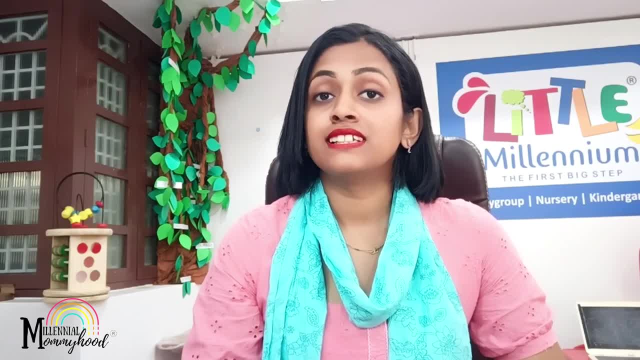 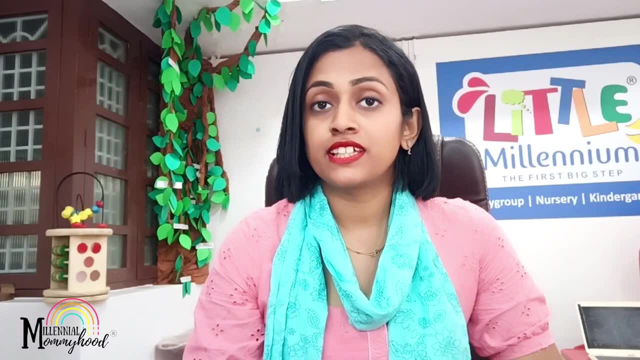 that out To make it very simple for you all. it is compulsory that the child have to be six years old in order to join first standard, So it is very easy to say that we can backtrace and check the age for which your child will be eligible to join any of the classes that you are. 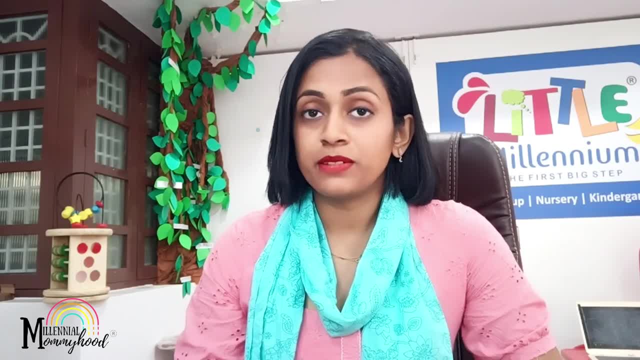 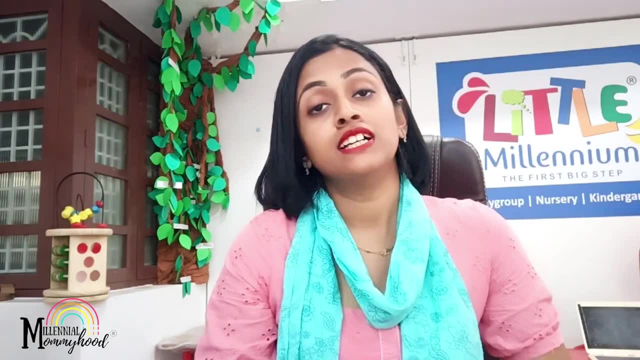 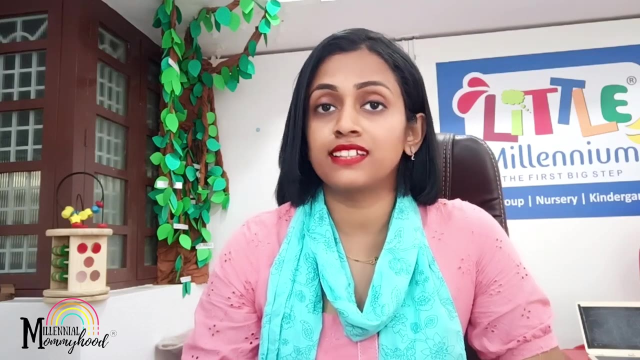 planning to send them to. So, according to NEP, if we backtrace, the age criteria is going to be as: two to three years going to pre-nursery or playgroup, three to four years going to nursery, four to five years going to LKG and finally five to six years going to UKG, and then they go turn six. 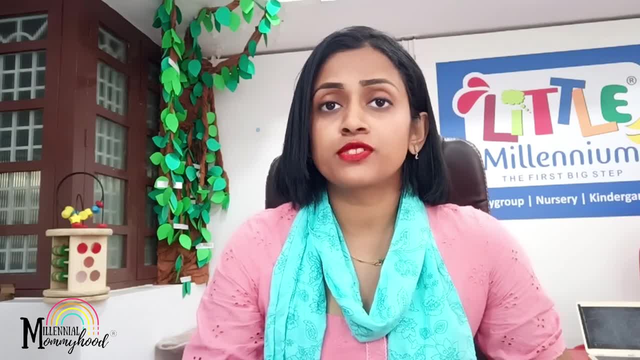 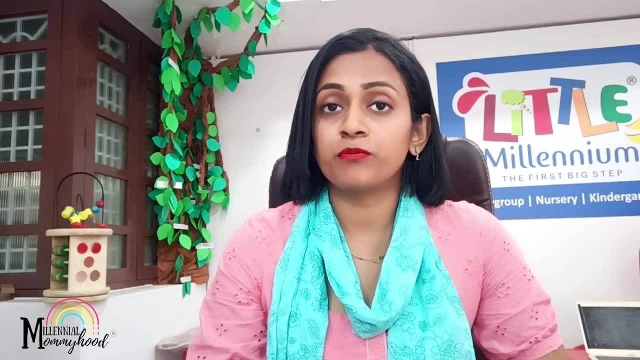 and then they go to first standard. Now, since majority of the schools are not taking children below six years old, even by a month, or even by a week, according to NEP- it is very important that we make sure that this criteria is met when you are taking admission for your child in any of the 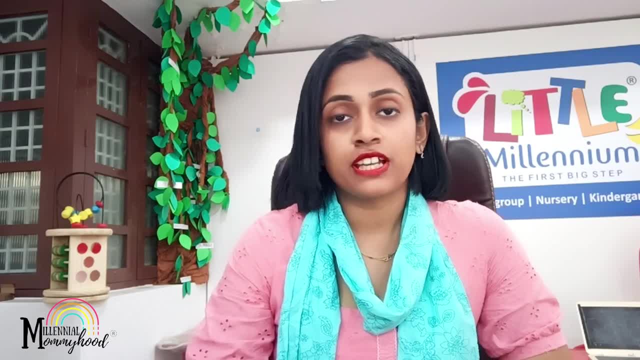 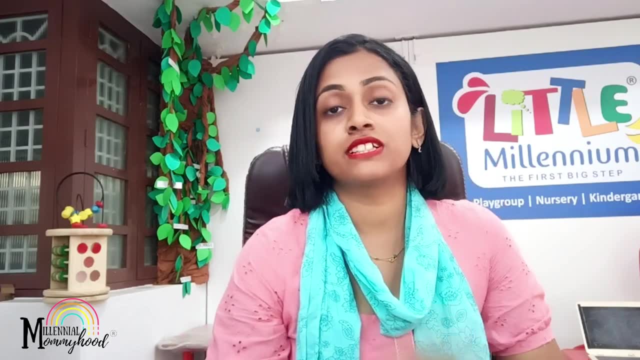 preschools. How to calculate that? Let me say your child is 3.1.. Now the child have completed three years, but the child have not completed four, which means your child clearly fits into the second category, that is, nursery, And this is how you select. 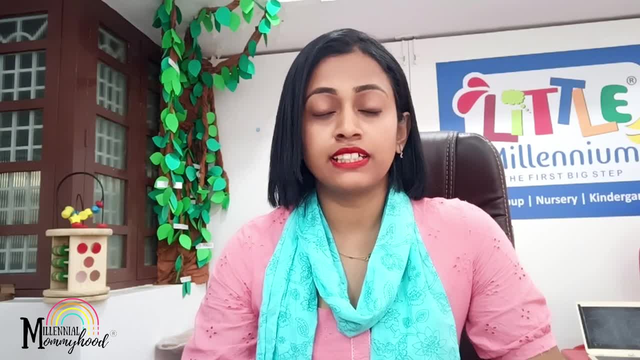 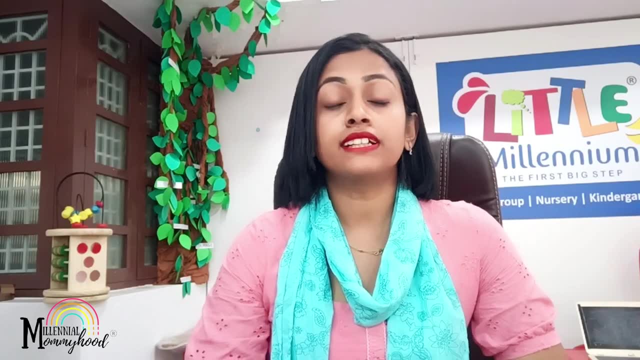 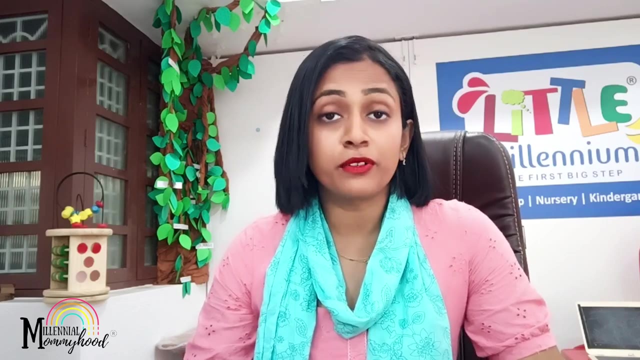 So if you have more doubts or confusions regarding NEP or anything related to age criteria, let me know in the comment sections and I'm going to definitely help you out. But though, it is your choice as a parent to decide whether your child have to go to a nursery, LKG, pre-KG or whatever.